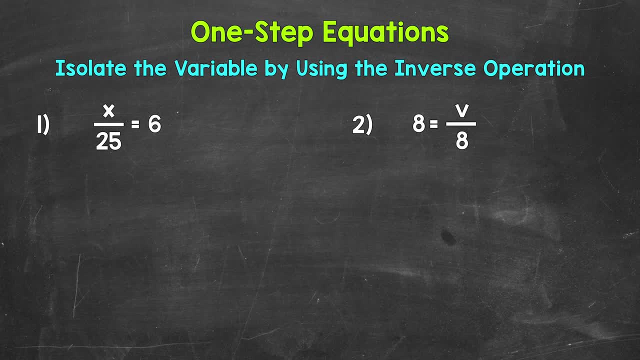 That keeps everything balanced and equal. Let's jump into number one, where we have x divided by 25 equals 6.. Now we need to isolate that variable of x. We need to figure out what x equals, Since x is being divided by 25,. 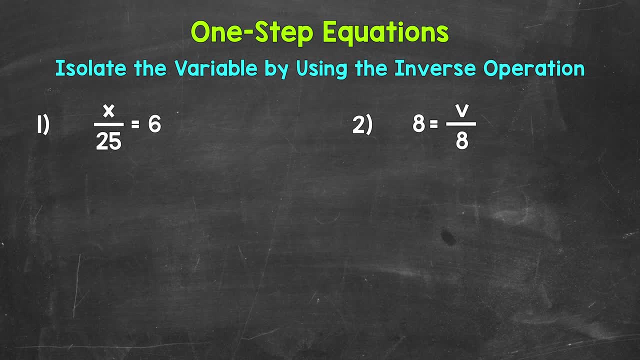 we need to undo that division by using the inverse operation. So the opposite operation, The opposite of division, is multiplication. So let's multiply the left side of the equation by 25.. Now, whatever we do to one side of the equation, 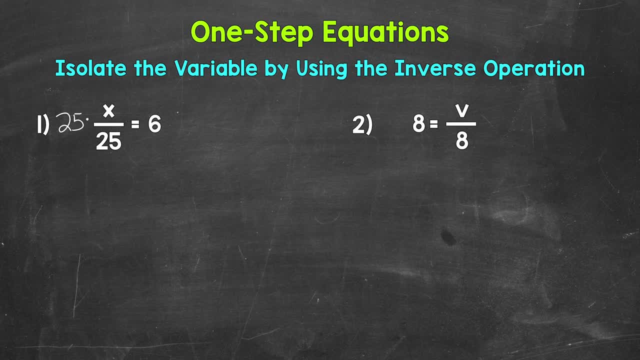 we must do to the other in order to keep it balanced and equal. So let's multiply the right side by 25 as well. Now let's take a look at the left side of the equation. We are dividing by 25 and multiplying by 25.. 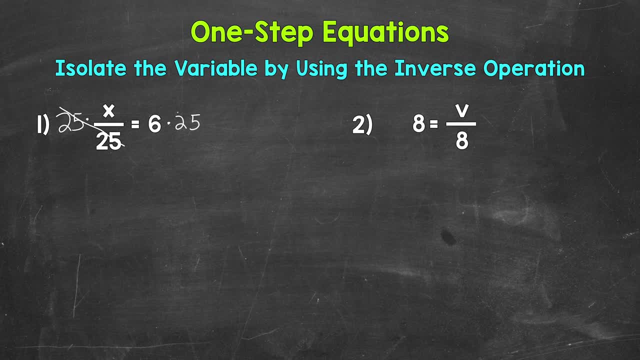 So these 25s cancel out. They equal 1.. Let's come to the side and quickly take a look at how the 25s cancel out and equal 1. We are multiplying x divided by 25.. So we have 25 times x divided by 25.. 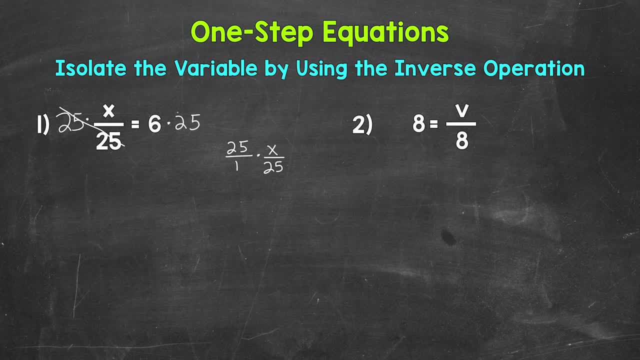 I wrote 25 in fractional form, since the division problem was in fractional form. That way we have numerators and denominators and we can multiply straight across. We are just multiplying fractions here. Remember, we can write any whole number in fractional form. 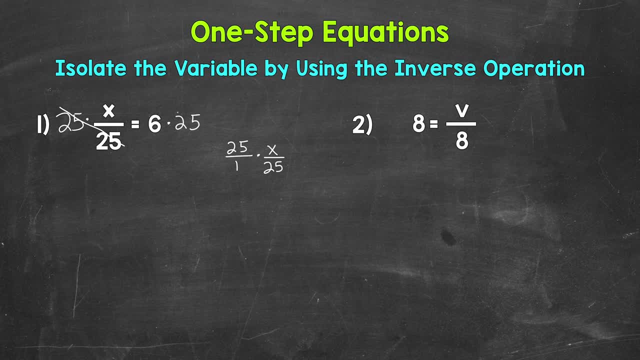 by putting it over 1.. Let's multiply. We'll start with the numerators. so the top numbers 25 times x, that equals 25x. Now we can multiply the denominators, so the bottom numbers 1 times 25,, that equals 25.. 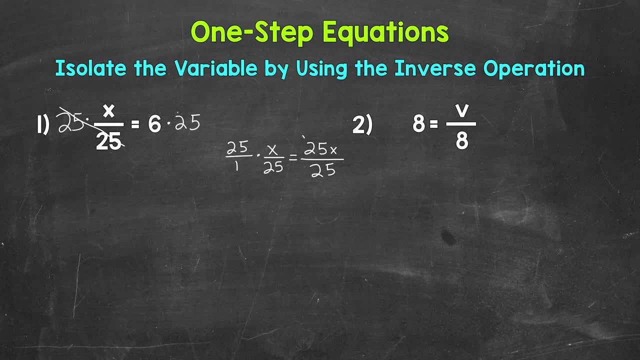 So we have 25x over 25.. These 25s cancel out. They equal 1.. We have 25 divided by 25.. That gives us that 1. So we have 1x, which is just x. 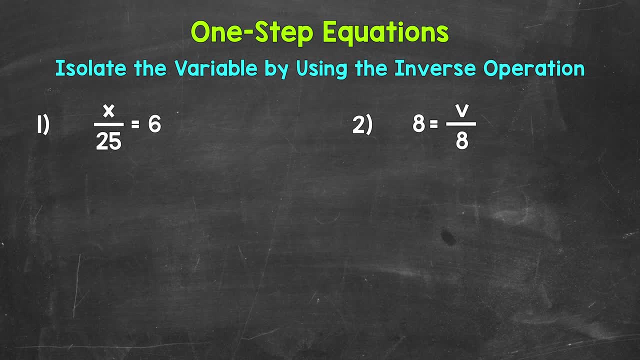 we need to undo that division by using the inverse operation. So the opposite operation, The opposite of division, is multiplication. So let's multiply the left side of the equation by 25.. Now, whatever we do to one side of the equation, 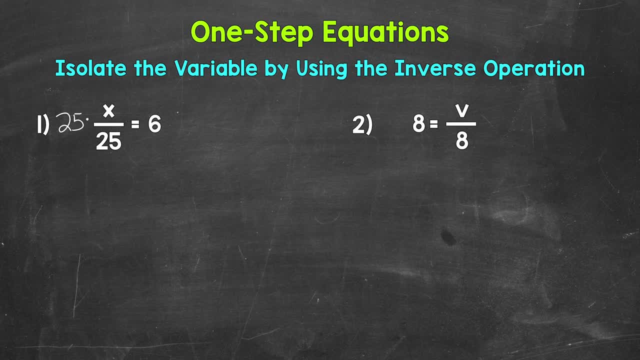 we must do to the other in order to keep it balanced and equal. So let's multiply the right side by 25 as well. Now let's take a look at the left side of the equation. We are dividing by 25 and multiplying by 25.. 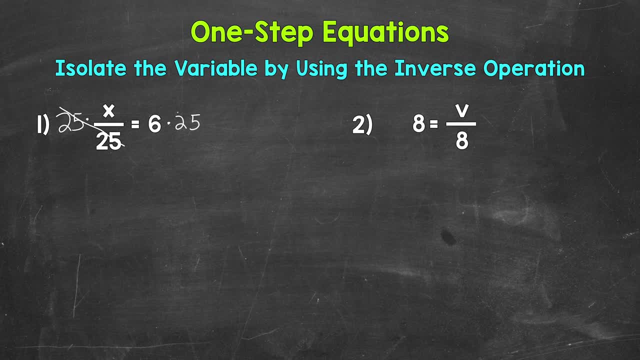 So these 25s cancel out. They equal 1.. Let's come to the side and quickly take a look at how the 25s cancel out and equal 1. We are multiplying x divided by 25.. So we have 25 times x divided by 25.. 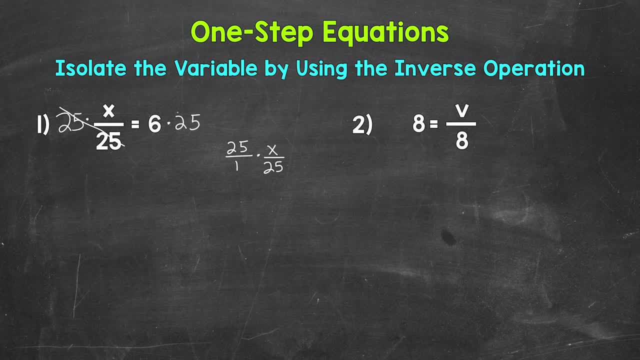 I wrote 25 in fractional form, since the division problem was in fractional form. That way we have numerators and denominators and we can multiply straight across. We are just multiplying fractions here. Remember, we can write any whole number in fractional form. 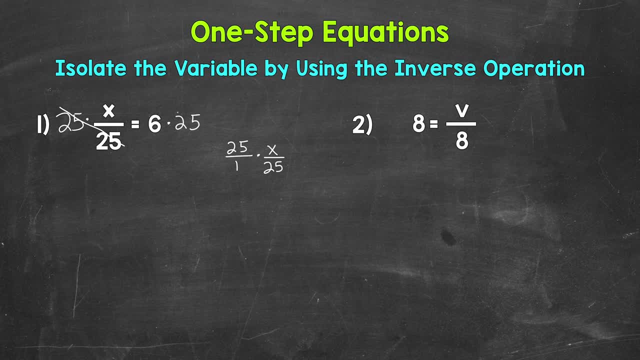 by putting it over 1.. Let's multiply. We'll start with the numerators. so the top numbers 25 times x, that equals 25x. Now we can multiply the denominators, so the bottom numbers 1 times 25,, that equals 25.. 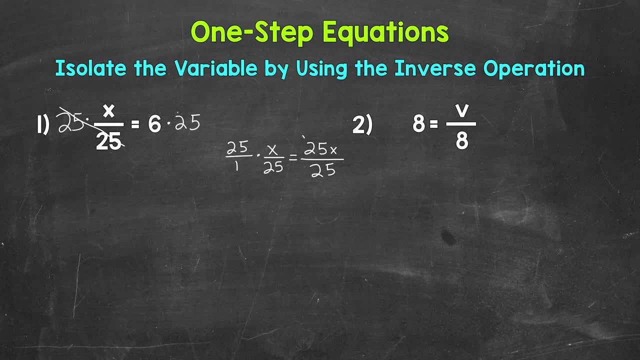 So we have 25x over 25.. These 25s cancel out. They equal 1.. We have 25 divided by 25.. That gives us that 1. So we have 1x, which is just x. 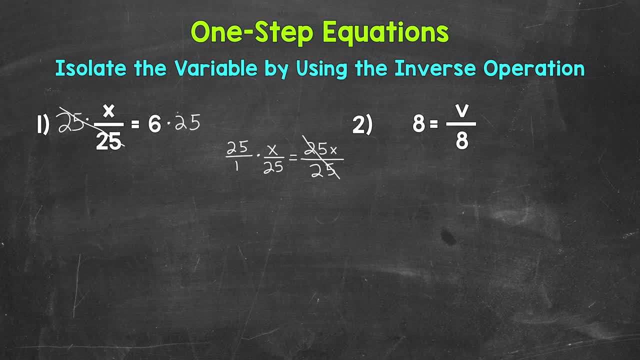 So the variable is now isolated, It's by itself. So we have x on the left side equals, and then on the right side 6 times 25.. That equals 150.. x equals 150.. That's our solution. 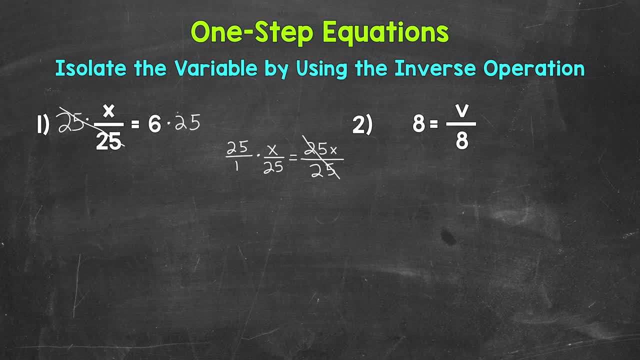 So the variable is now isolated, It's by itself. So we have x on the left side equals, and then on the right side 6 times 25.. That equals 150.. x equals 150.. That's our solution. 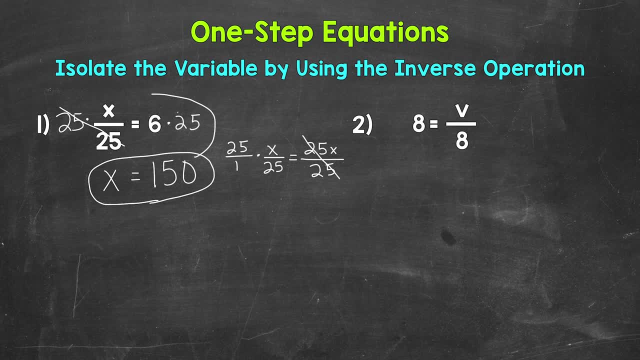 Now we can always check a solution by plugging it into the original equation. So let's plug 150 in for x and see if this works. 150 divided by 25 equals 6.. 150 divided by 25 does equal 6, so that's the correct solution. 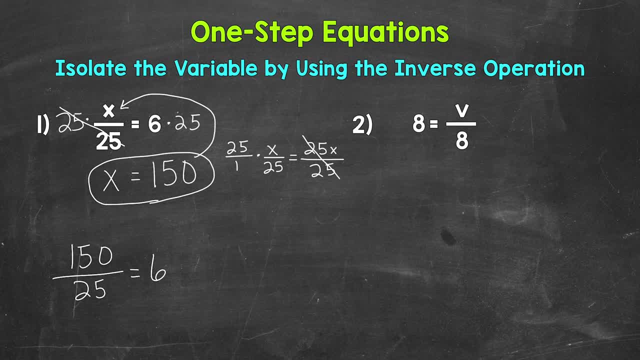 x equals 150.. Let's move on to number 2, where we have 8 equals v divided by 8.. Now we need to isolate that variable of v. v is being divided by 8. So we need to undo that division by using the inverse operation. 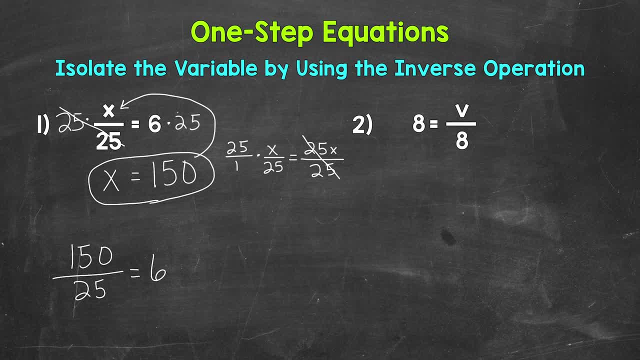 The inverse of division is multiplication. So let's multiply the right side of the equation by 8.. Now, whatever we do to one side of the equation, we must do to the other. So we need to multiply the left side of the equation by 8 as well. 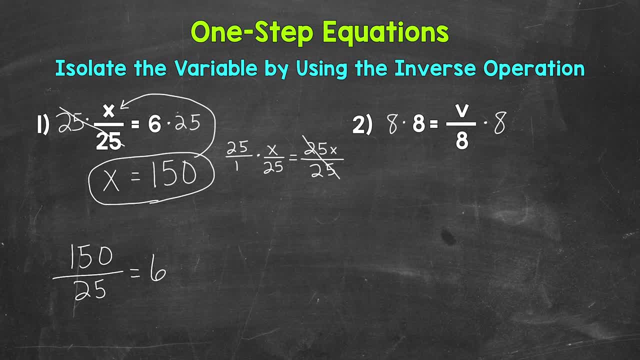 Now let's take a look at the right side of the equation. We are dividing by 8 and multiplying by 8. So these 8s cancel out. They equal 1. That gives us 1v, which is just v. 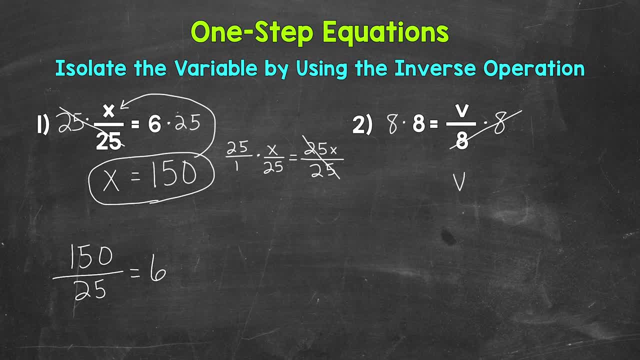 So the variable is now isolated. v equals and then, on the left side of the equation, 8 times 8. That equals 64. So v equals 64. And we can rewrite this with the variable coming first. Let's check that solution by plugging 64 in for v in the original equation. 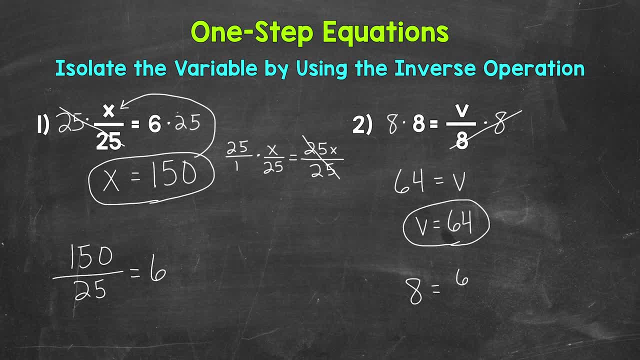 So we have: 8 equals 64 divided by 8.. 64 divided by 8 does equal 8.. So that's the correct solution: v equals 64.. So there you have it. There's how you solve one-step division equations. 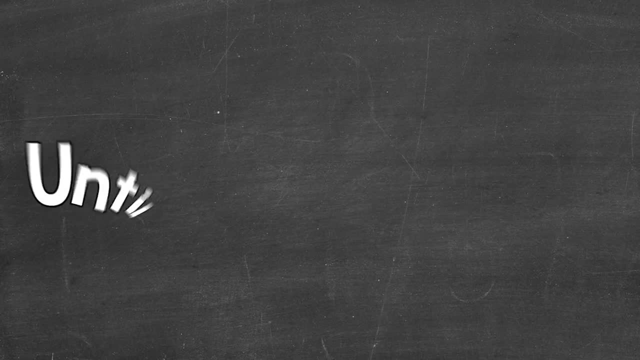 I hope that helped. Thanks so much for watching. Until next time, peace.